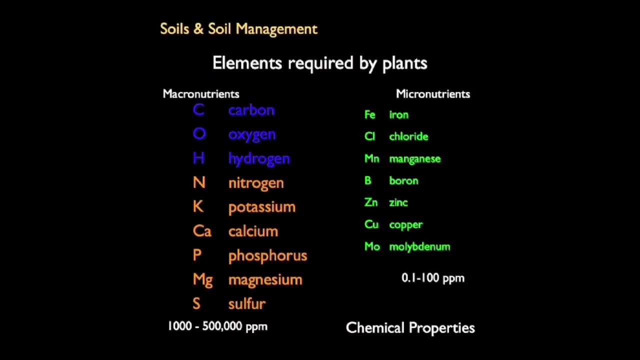 Of the elements listed here, macronutrients such as carbon nitrogen, phosphorus and potassium are needed in quantities generally between 1,000 and 500,000 parts per million, whereas micronutrients such as iron, manganese and zinc are required in much smaller quantities. 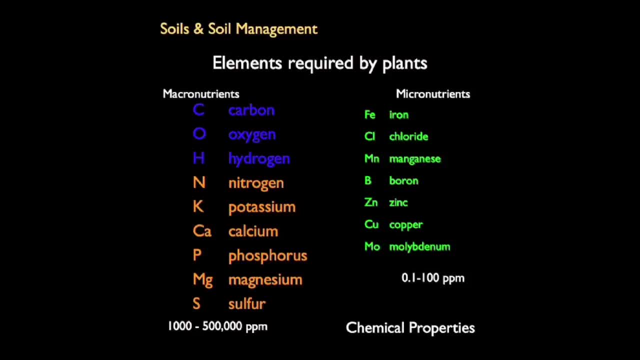 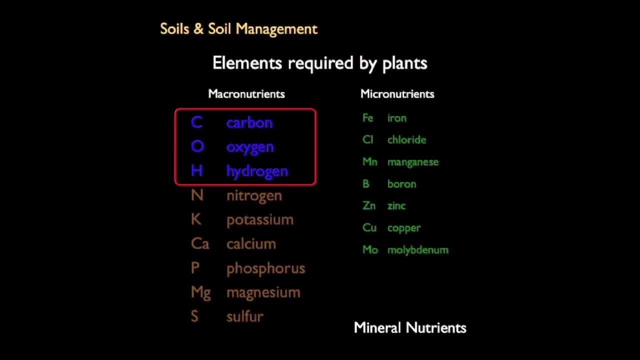 of about a tenth to 100 parts per million. Carbon, oxygen and hydrogen are considered the non-mineral nutrients of plants, as they are primarily obtained from the air and water. The rest of the nutrients are considered mineral nutrients and they are derived exclusively. 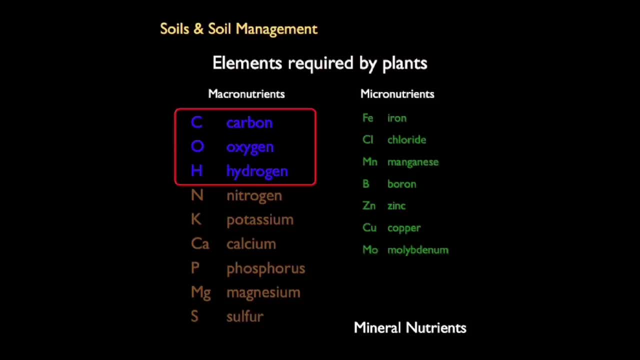 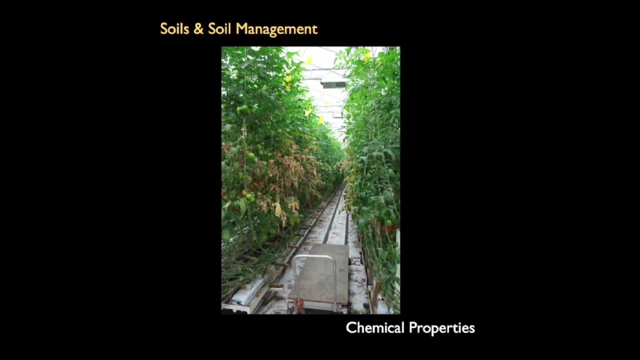 from the soil. Thus, an understanding of soil chemistry is essential for an understanding of plant growth and development. It is interesting that most of the mineral and organic components of soil contribute to its bulk and structure, but these components cannot be used directly or are not used directly. 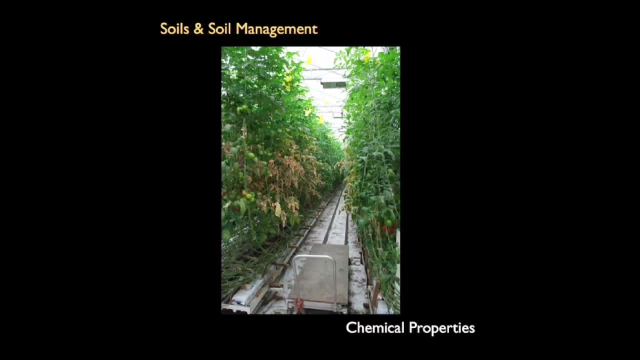 or are not required by plants. Consider, for example, that these tomato plants are being grown without any soil in artificial systems described as hydroponics. Plants obtain their mineral nutrients from a relatively small fraction of the soil that is in solution on the surface of soil particles. 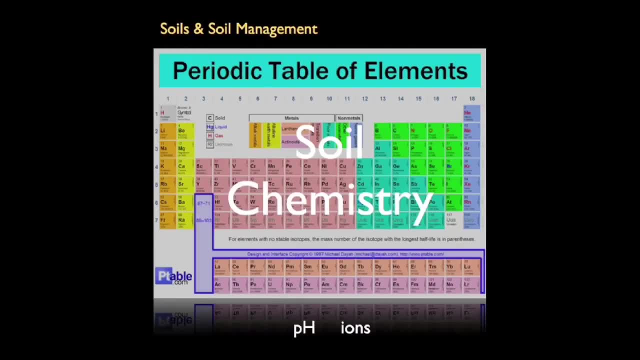 In this section on soil chemistry, I will present topics that deal with soil pH And the key nutrient elements that plants obtain from soil. You will see that the pH of the soil solution varies from about 3.5 to 8.5,, but most plants 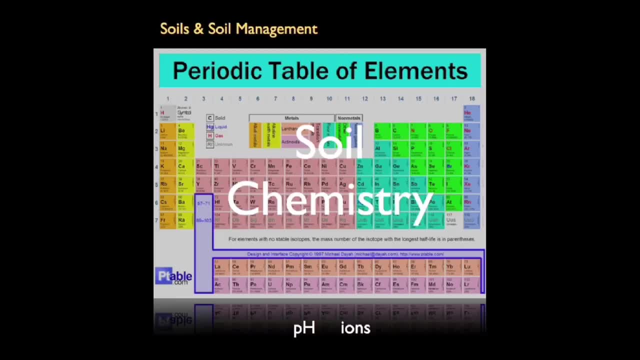 can only grow in soils between pH 6 and 7.. The nature of the parent material, the activity of soil organisms and the amount of precipitation influences soil pH. With respect to mineral nutrients, you will see that nitrogen is often the limiting nutrient. 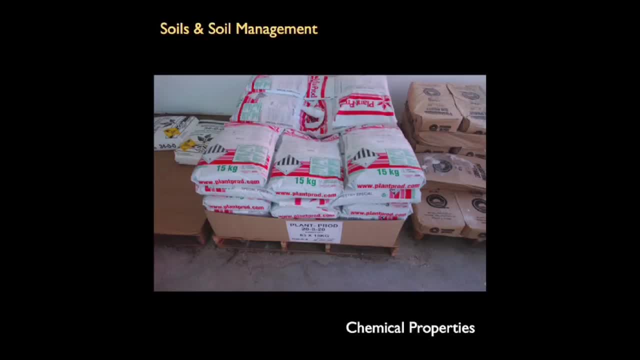 for plant growth. Nitrogen is often the limiting nutrient for plant growth. Nitrogen is often a very significant nutrient for plant growth. Nitrogen is often the most important nutrient for plant growth. Nitrogen is an essential ingredient and can be used for a lot of other things. 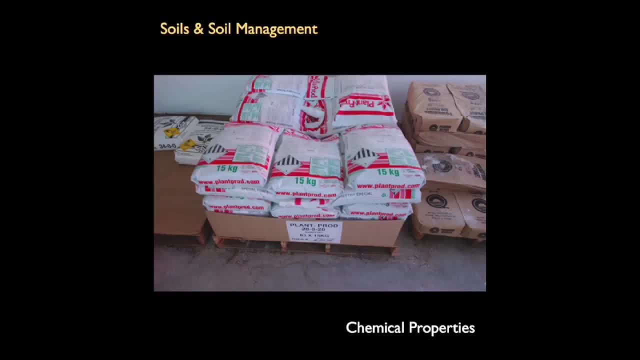 Nitrogen is a substitute for soil resistant materials such as sediments, pectin and other compounds, But this chemical is often not applied to soil in several forms In most other situations where we grow plants, either agronomic crops, turf for golf courses- 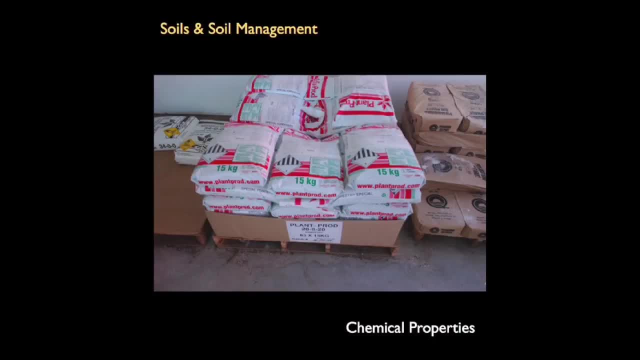 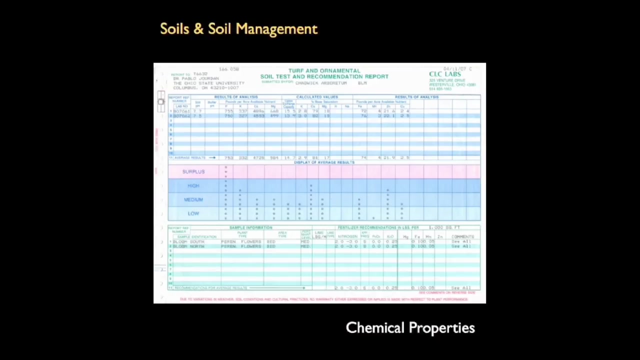 landscape trees or shrubs and greenhouses plants. many other chemicals are added to soils or to media to supply particular nutrients or to modify soil pH. A direct application of soil chemistry knowledge is a soil test. Testing the soil is a standard best practice. 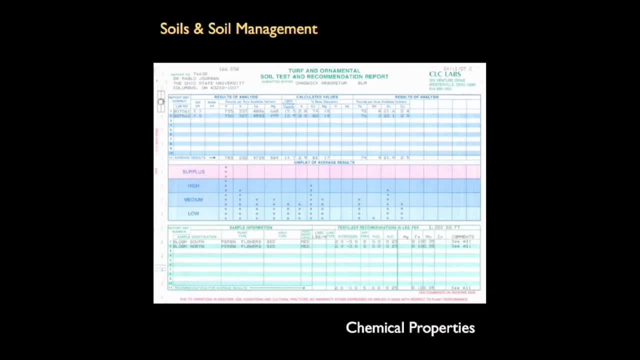 Soil tests provide scores of soil tests provide scores of soil areas of crop agriculture, including turf and landscape. The key information provided by a soil test is about the chemistry of the soil, such as the pH, the concentration of key nutrients and the cation exchange capacity. More on these terms later. 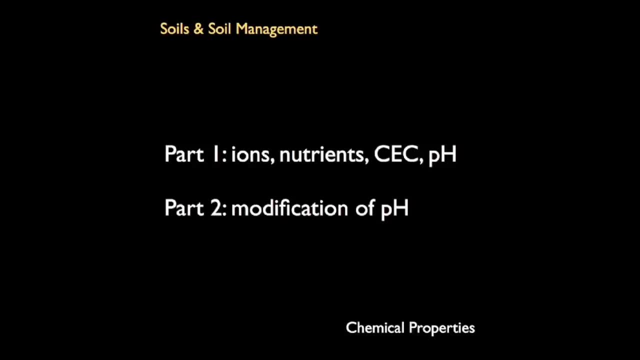 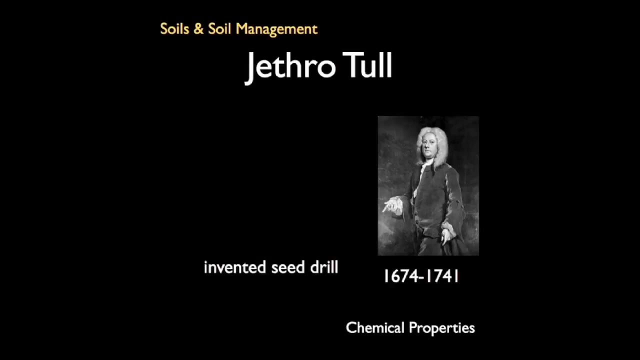 This unit on the chemical properties of soil is divided into two parts: one dealing with ions, nutrients, the cation exchange capacity and pH, the other with modification of soil pH. Now let us start with a bit of history. In 1731, Jethro Tull, an English farmer, inventor. 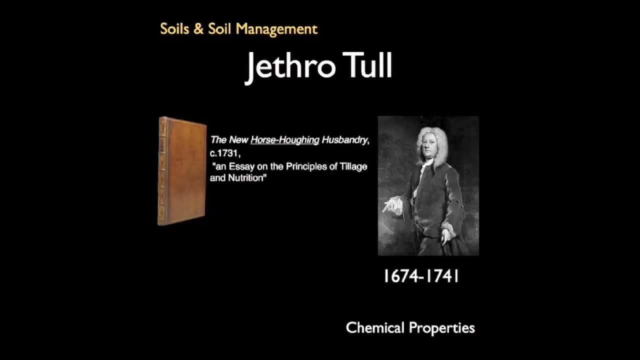 and author published an agricultural treatise entitled Horse-Hoeing Husbandry. In this manuscript, he maintained that plants survived and grew as a result of the soil. In this manuscript, he maintained that plants survived and grew as a result of the soil. 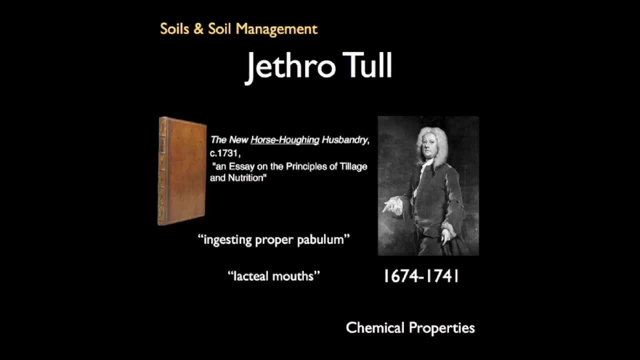 In this manuscript he maintained that plants survived and grew as a result of the soil. He thought that the soil was an excellent source of nutrients. It was a natural nutrient source, but it was not a very practical source. He found that the soil derived nutrients, as with the natural environment, by directly. 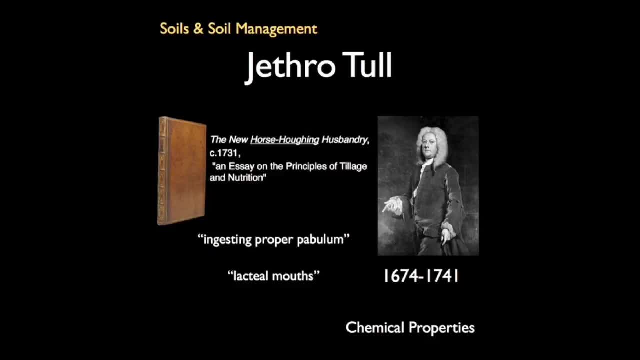 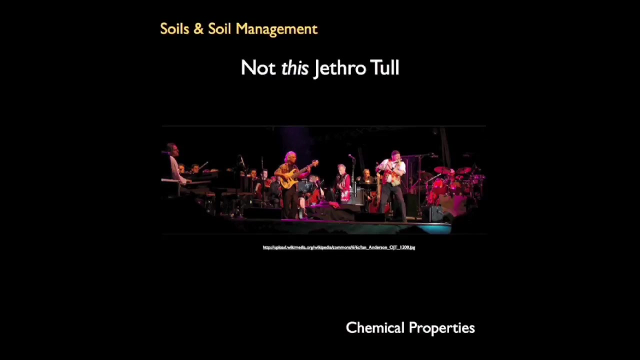 ingesting fine soil particles through root pores. Although his proposed mechanism for nutrient uptake was in error, he did correctly identify the soil colloids as important soil constituents affecting plant nutrient availability. They do so by virtue of their inherent chemical properties. Now, just in case you were wondering, we are dealing with a different Jethro Tull than 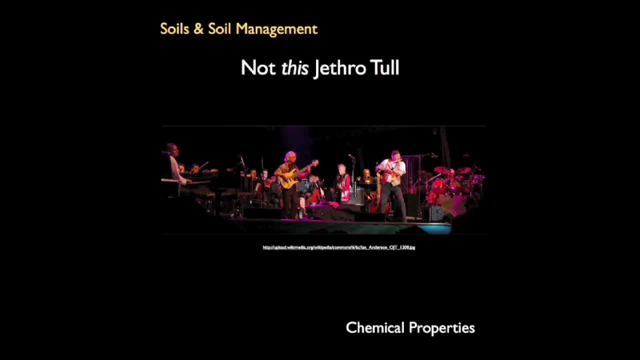 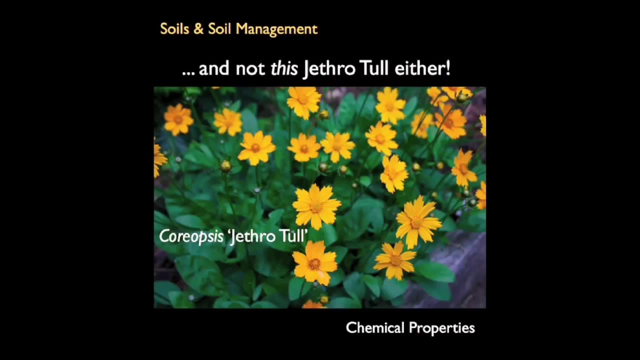 the popular British rock group from the 1970s and 80s. although the band is named for this famed British agriculturist, There is also a popular ornamental plant, the Tixeed or Coreopsis Jethro Tull, introduced by Itzol Plants and patented. Imagine using this plant in combination with 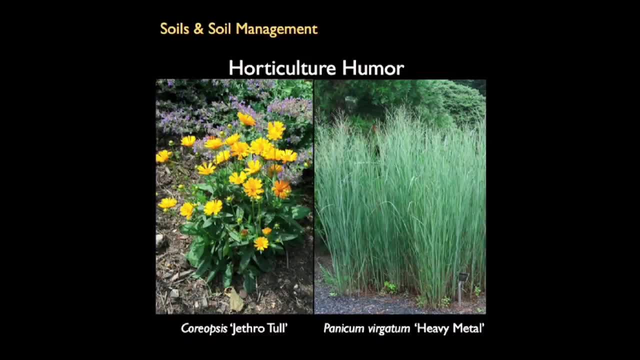 another wonderful ornamental switchgrass named Heavy Metal. Now who says horticulturists don't have a sense of humor. But I digress. The chemistry of soils is important and a somewhat complex material, But its importance cannot be under-emphasized. A key concept to keep in mind is that elements 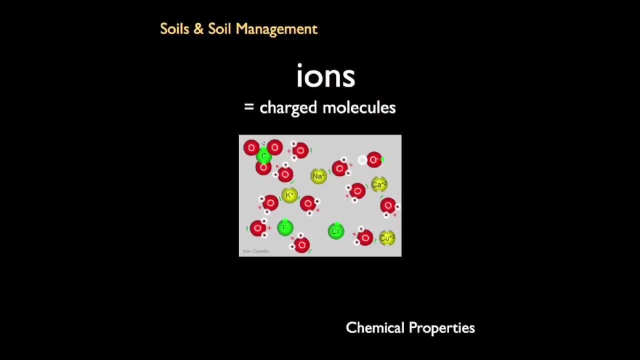 involved in various soil chemical processes are charged molecules. They are ions. Positively charged ions are called cations. for example, hydrogen, potassium and magnesium Cations are the key components of the cation exchange capacity, an important characteristic of soils. 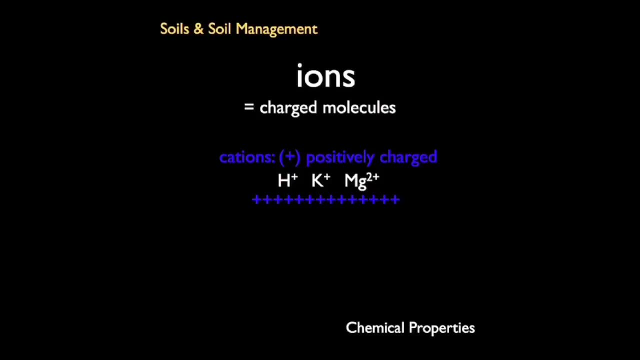 But it is not always the case that the cations are charged. The cations are charged by the same result between theoud, potassium, calcium and magnesium. The ions are major plant nutrients that occur as positively charged ions. They can be held together in negatively charged. 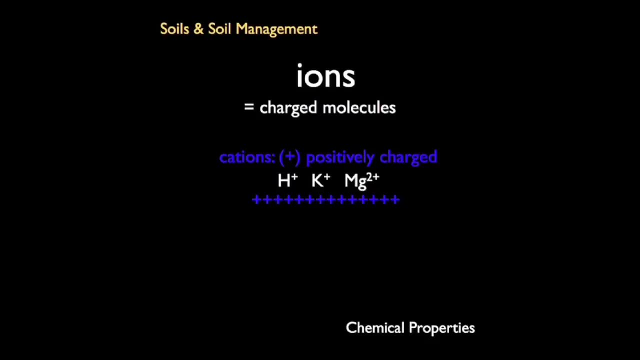 groups on particles of mineral and organic matter and released relatively easily for uptake by the plant. Negatively charged elements are called anions, such as hydride, chlorine and phosphate ions shown here. Cations and anions are influenced by acid-base theory. 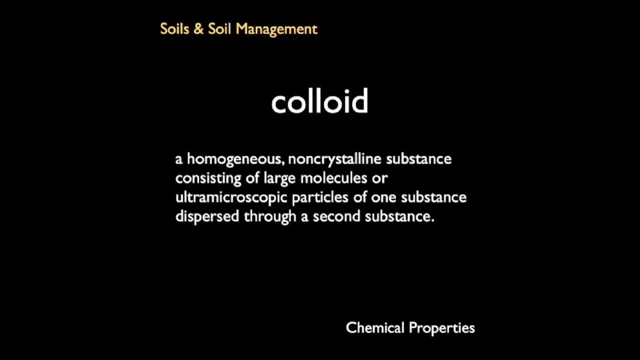 of general chemistry. In the definition of soil, we saw that it exists as an unconsolidated, porous medium. Essential physical components of soil behave as colloids, and a colloid is defined as a homogenous, non-crystalline substance consisting of large molecules or 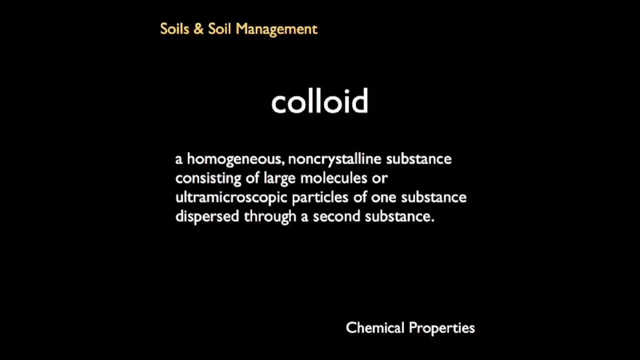 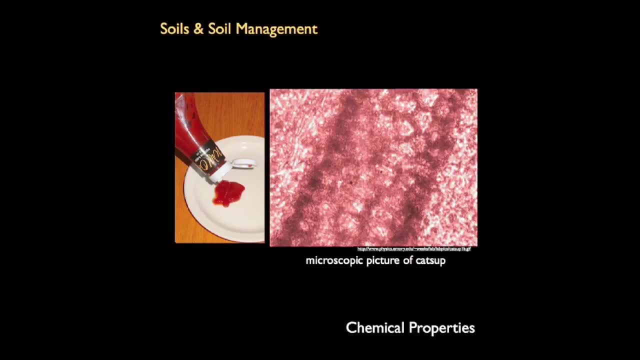 ultra-microscopic particles of one substance dispersed through a second substance. Colloidal materials are small, often electrically charged amorphous solids that are suspended or dispersed in a liquid medium. Ketchup is a good example of a colloidal suspension In ketchup pureed. 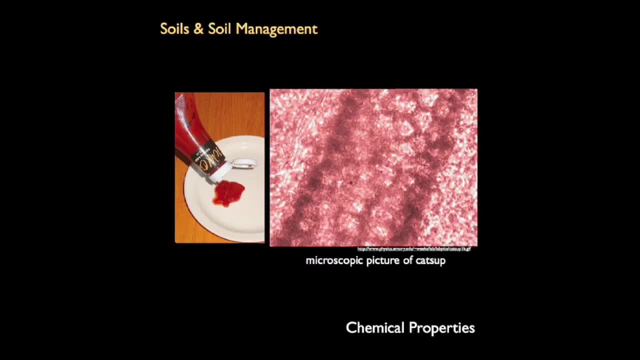 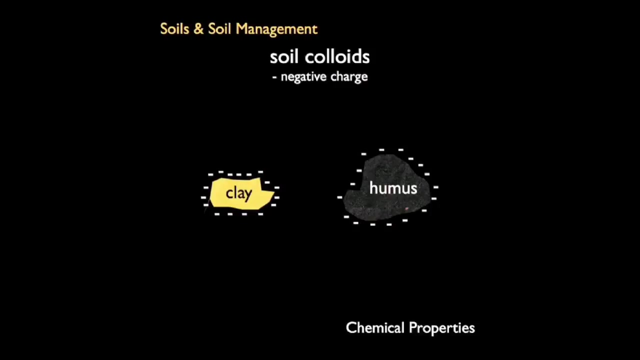 tomato particulates are dispersed within a liquid medium containing water, sugar, vinegar, salt, spices and flavorings. Repelling forces between particulates themselves and with the liquid medium keep them from coalescing. Clay and humus particles are quintessential colloidal materials. They are small usually. 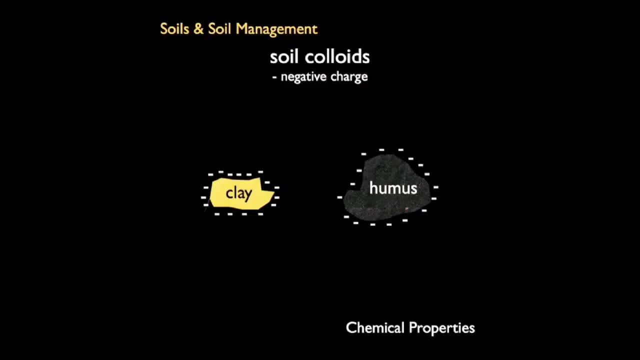 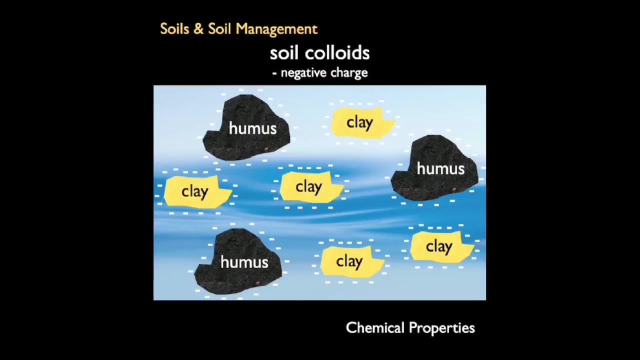 about 2 micrometers in diameter. They have a high surface-to-volume ratio. They exhibit a net electrical charge that is usually negative. Finally, because they are charged, they repel one another and can easily be dispersed in the soil solution. 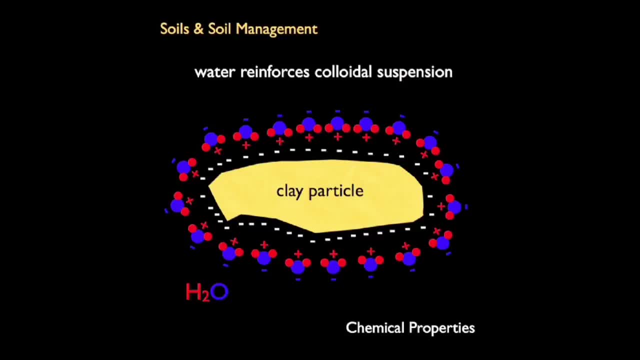 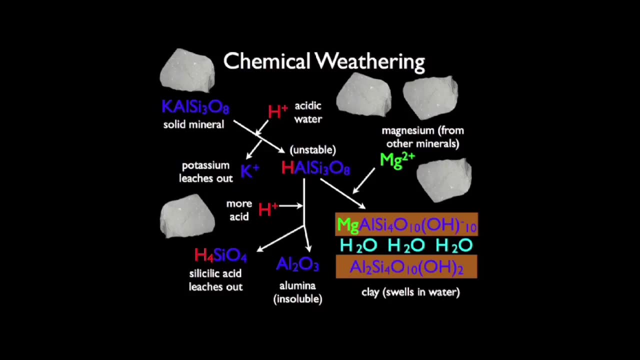 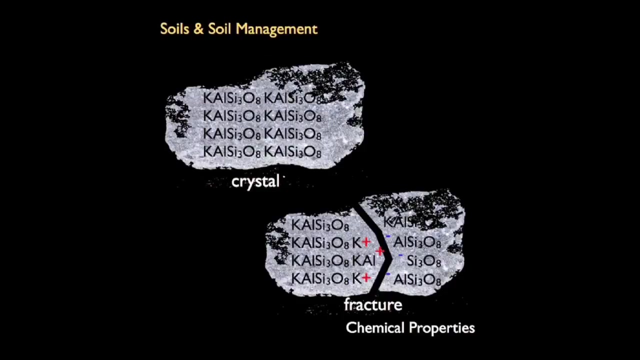 The virtue of its polarity, actually reinforces the colloidal suspension. As we saw, soil particles are formed by weathering of rock minerals. The weathering changes their crystalline structure and alters their electrical charge. Sometimes the fracturing of mineral particles can separate charges on the resulting fragments. 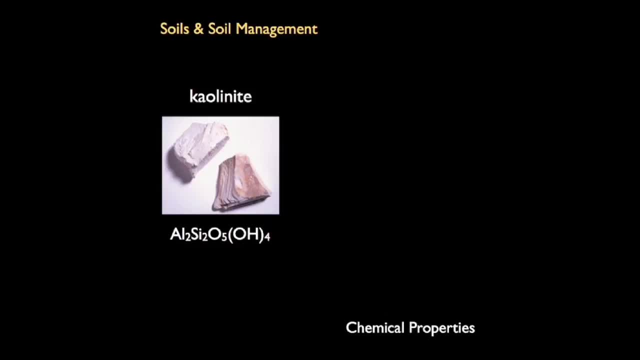 Aluminosilicate clays account for most of the charged particles in mineral soils in the temperate zone. They come in a variety of materials such as kaolinite, illite and montmorillonite. Kaolinite is a clay mineral with a chemical composition shown here: Rocks. 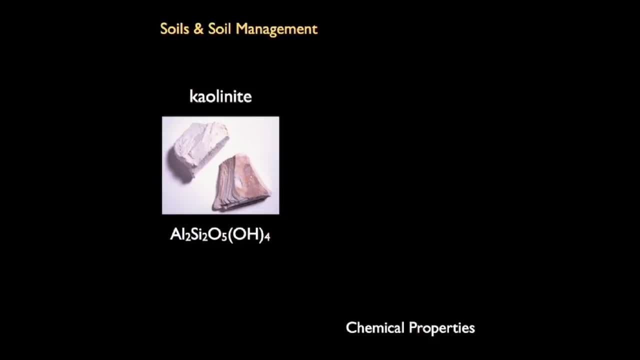 that are rich in kaolinite are known as china clay or kaolin. While these minerals are important for the development of soil and influence the role of soil in supporting plant growth, it is interesting to know that these materials also have other functions that are indirectly 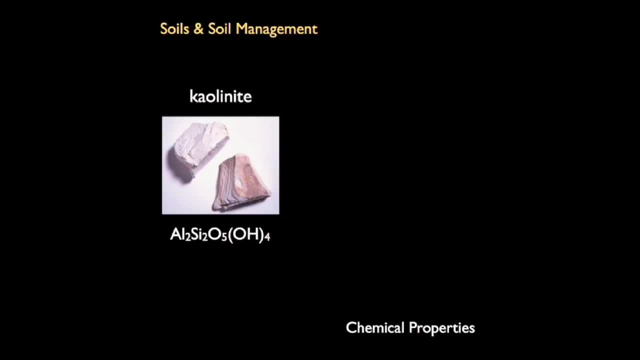 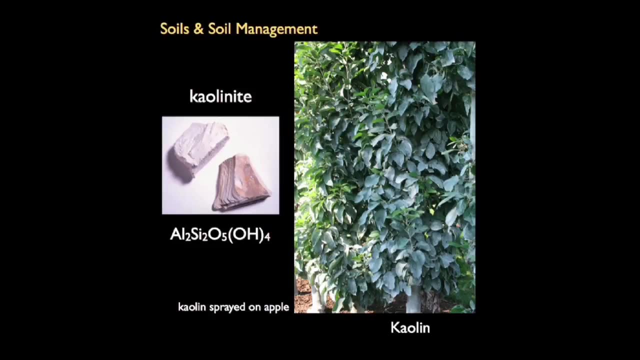 relevant for the modern growth of plants. For example, a more recent and more limited use of kaolinite is as a specially formulated spray applied to organic fruits, vegetables and other vegetation that coats the surfaces with a white residue and seems to repel, or. 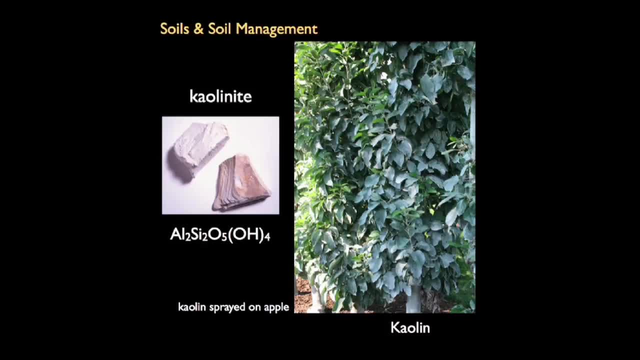 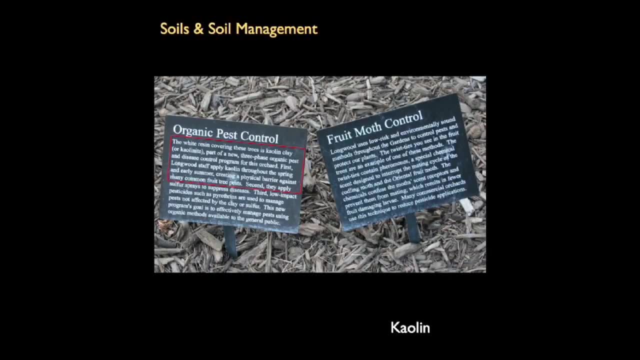 deter insect damage. The use of kaolinite is a special form of a chemical that is used to prevent direct damage and, at least in the case of apples, to prevent sun scald. Kaolinite is applied throughout the spring and early summer, creating a physical barrier. 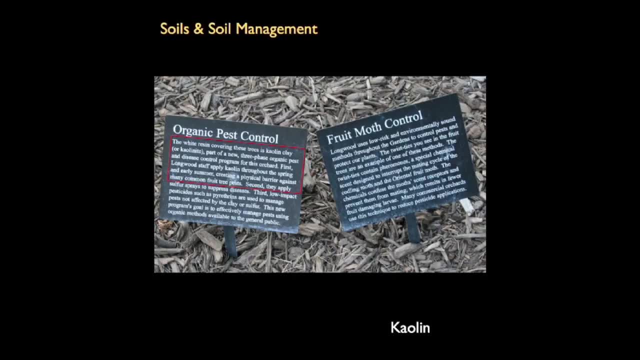 against many common fruit tree pests. The label from this educational garden display reads: the white resin covering these trees is kaolin clay, part of a new three-phase organic pest and disease program for this orchard Kaolin is used in ceramics medicine. 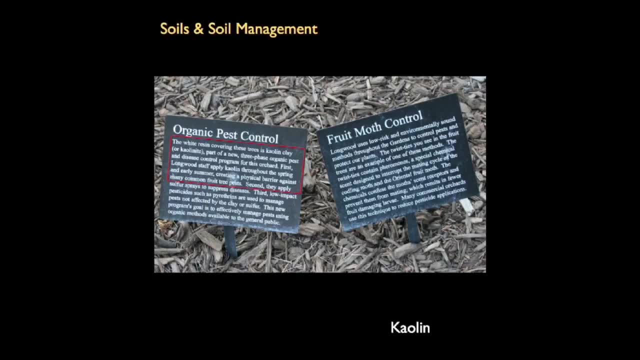 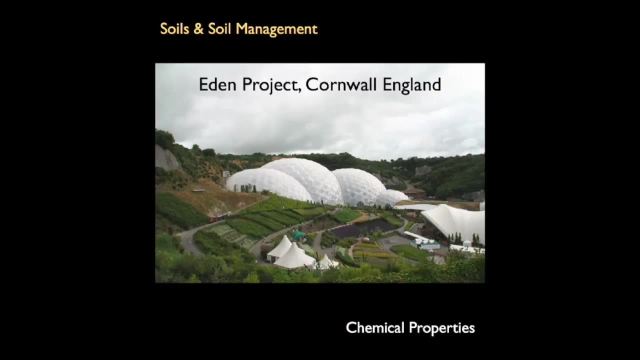 laboratory and the use of food products, such as food products and natural materials. Kaolinite is used as a food additive, a toothpaste, a light diffusing material and as a white incandescent light bulb. It is generally the main component of porcelain. The region. 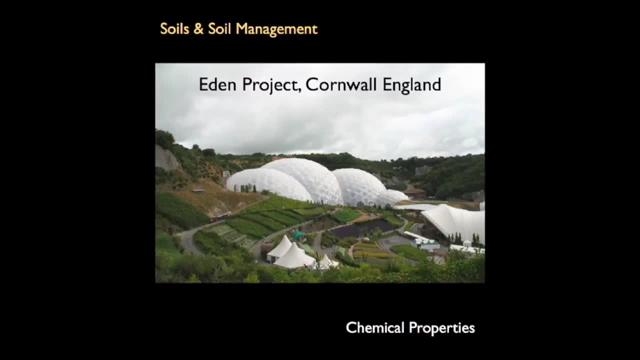 of Cornwall in England is known for its abundant clay mine and the porcelain derived from it. Interestingly, the largest greenhouses in the world. part of the Eden Project, a large environmental complex near St Austell in Cornwall is constructed. The greenhouses are designed. and built to create a space for the use of food products and other natural resources, and then for the use of natural resources such as food: Kaolinite is used as a food additive, toothpaste as a light diffusing material, in white incandescent light bulbs and in cosmetics. 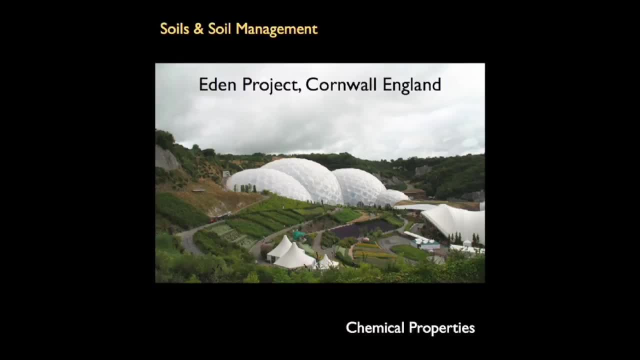 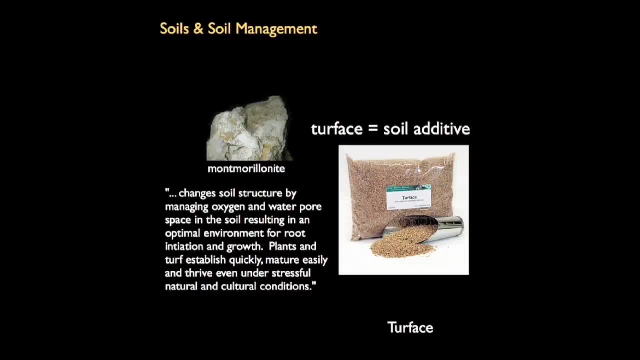 It is generally the main component of porcelain. The region of Cornwall in England is known for its abundant constructed in a disused china clay or kaolin pit. Still another example of horticultural use of these special materials is turface. Montmorillonite can be baked to produce. 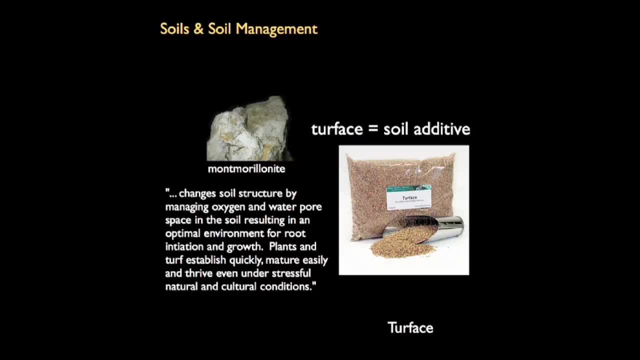 arcelite, a porous calcined clay sold as turface products, a soil conditioner for playing fields. These are touted to have great properties, as described here. Changes soil structure by managing oxygen and water pore spales in the soil, resulting in an optimal environment for root. 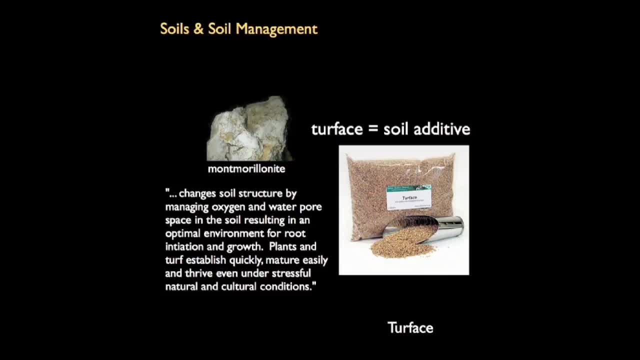 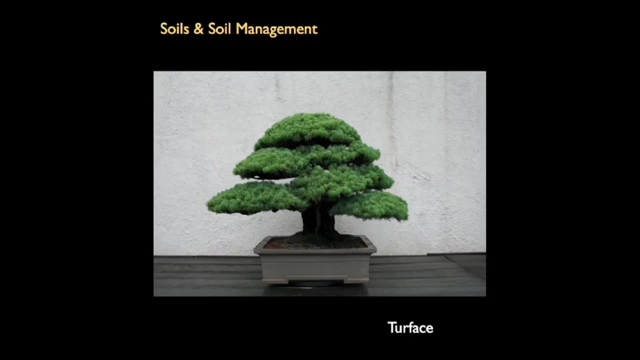 initiation and growth. Plants and turf establish quickly, mature easily and thrive even under stressful natural and cultural conditions. You can see, this is a great marketing material. Now turface is also very popular as a bonsai soil, used very extensively for these wonderful art forms. 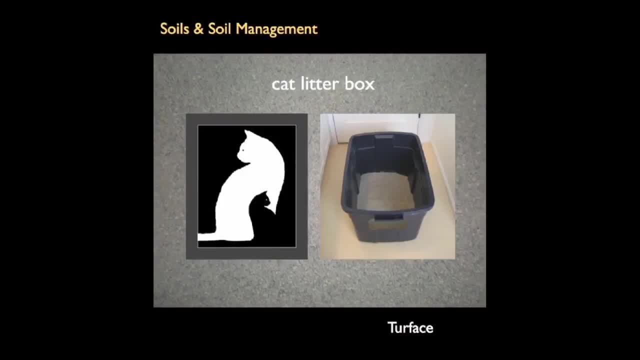 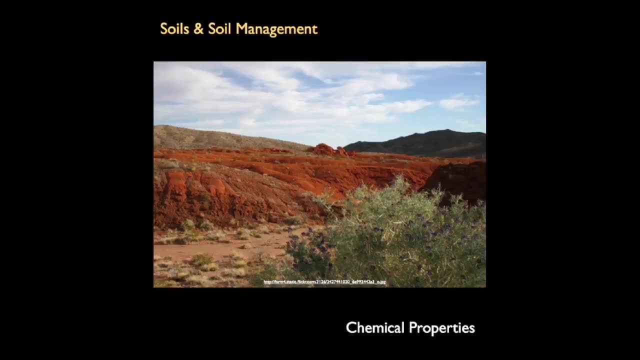 Finally, cat litter is also made out of this similar material, like turface. Now still another class of clays. the hydrous oxide clays are interspersed with aluminum silicate clays in temperate zones, but are major soil minerals in the tropical and semi-tropical regions. The red color of soils is 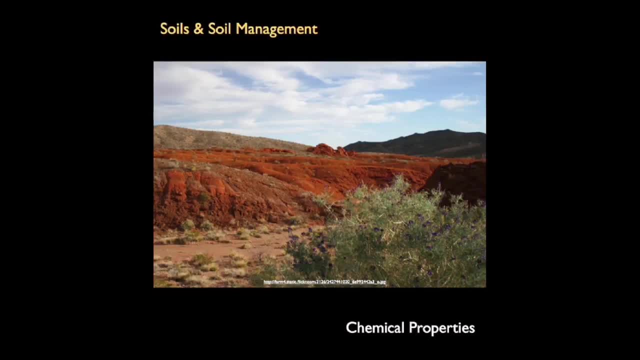 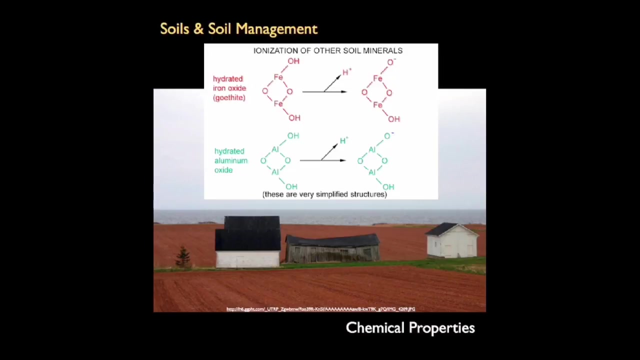 generally related to unhydrated iron oxides, although manganese dioxide and partially hydrated iron oxides may also contribute red colors. Since unhydrated iron oxide is relatively unstable under moist conditions, red color generally indicates good drainage and good aeration. These iron or aluminum based colloids are highly hydrated and can become negatively charged if hydroxyl groups within the lattice become ionized. 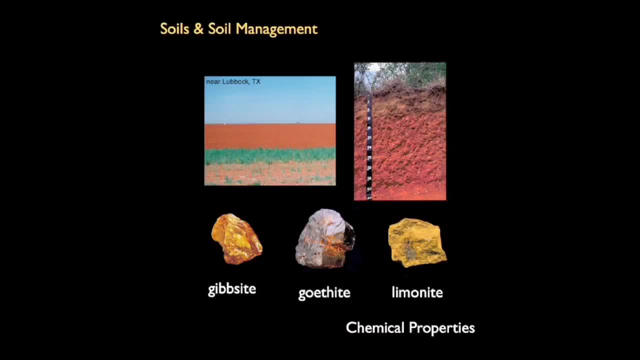 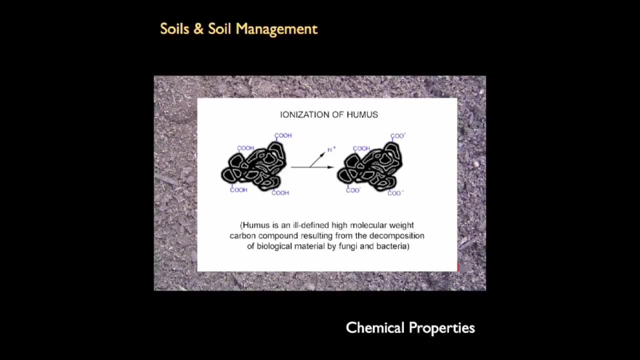 Examples of these clays include gibbsite, gethite and limonite. Now, after soil organisms have worked on organic debris in the soil, a complex, insoluble but hydrated material called humus remains. Much of this is in minute colloidal fragments adhering to mineral particles. 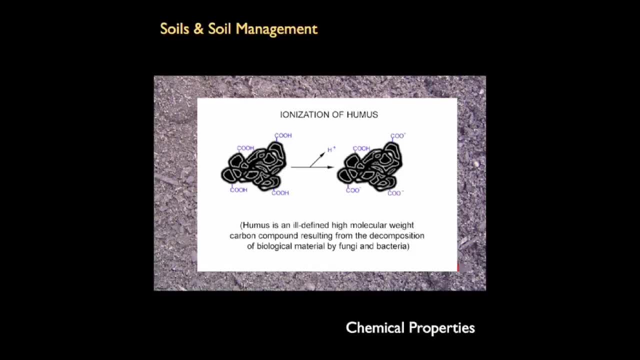 It is difficult to define the chemical structure of humus, but it is often weakly acidic and is then called humic acid. Like many other organic acids, including acetic acid, and in vinegar, it has carboxyl groups with the structure of humus. 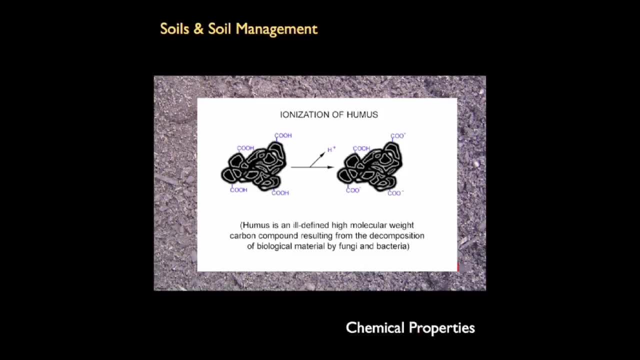 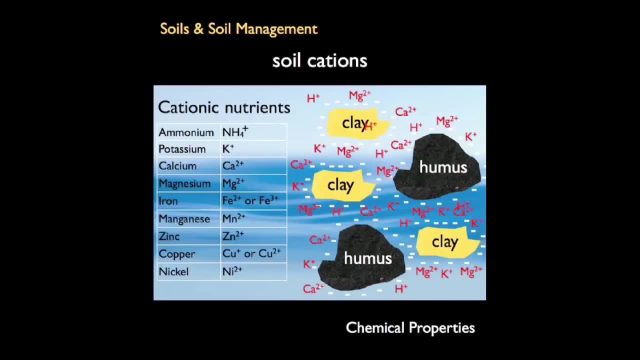 As if it were a liquid. the sitting particles of humus commit to getting rid of the effluent. This is an important factor in the development of organic and inorganic molecules and the involvement of this will be important. Organic and inorganic molecules are dissolved in this. 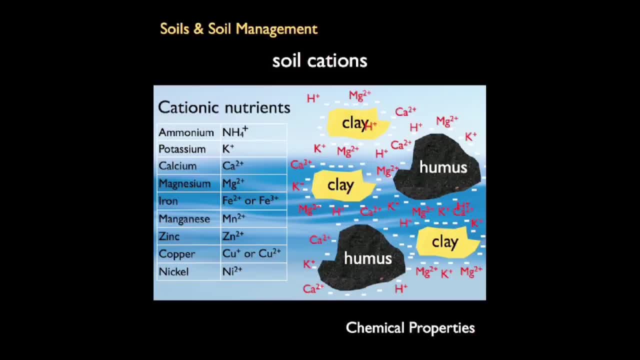 Inorganic salts tend to ionize in solution and some of the ions are nutrients that are immediately available to plants. However, most of the cationic or positively charged nutrients are held in loose association by the negatively charged soil colloids. The free and bound cations are in equilibrium, so that if some are absorbed by the plant, 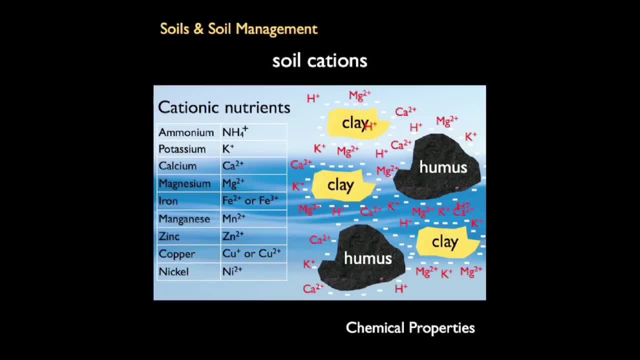 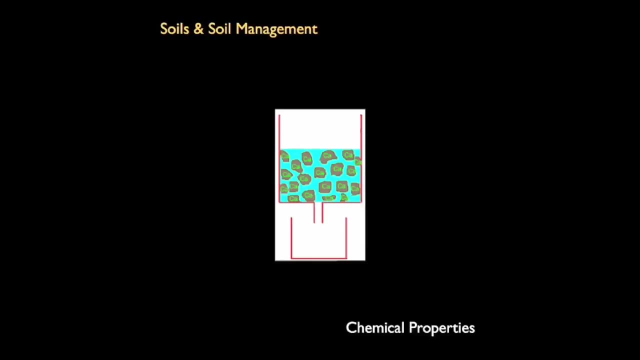 root, others will tend to come off the particles into solution. Therefore soil colloids act as the plant's bank account or storehouse for these nutrients. Cat ions loosely bound to the colloids and free ions in the soil solution can be exchanged for one another. 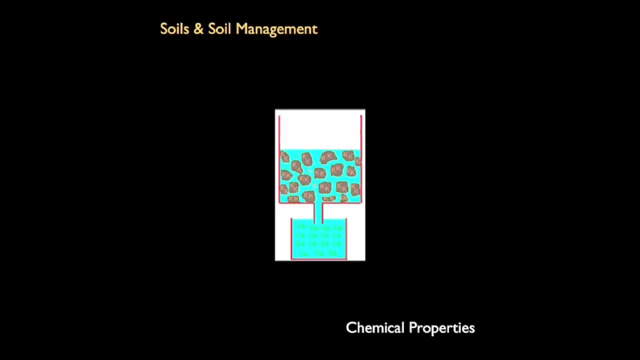 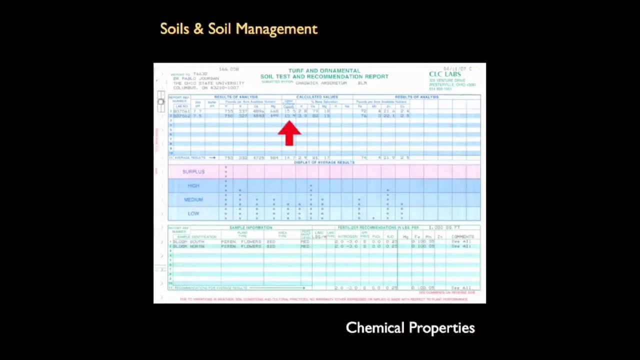 For example, potassium ions in solution could exchange for calcium on a soil particle. The holding capacity for nutrient ions is measured in cations In standard soil tests and reported as CEC or cation exchange capacity. this is an important measure because the exchangeable ions are available to plants supplementing the small. 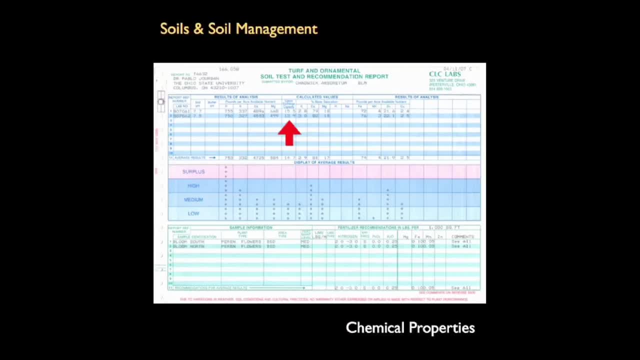 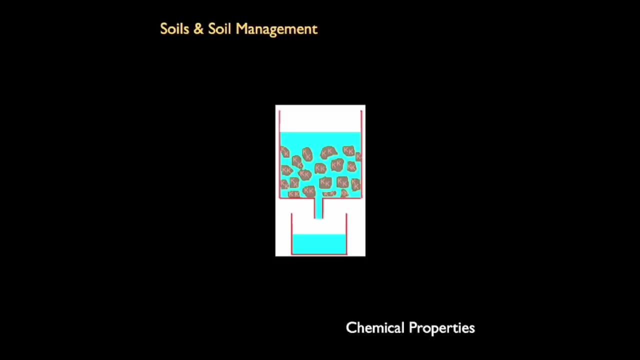 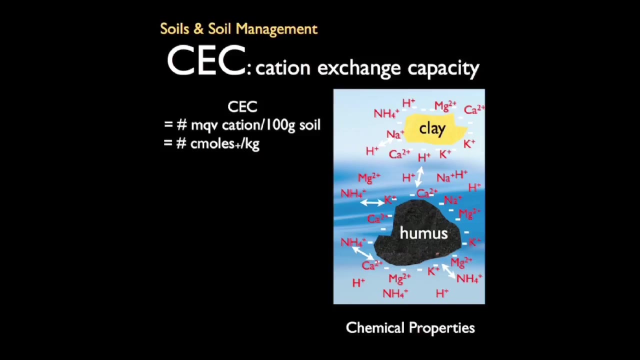 quantity in solution at a given time. Also, CEC helps retain nutrients in the soil. If they are bound to soil particles, the cations will not be so easily leached by rain or irrigation water. As indicated, An important property of clay and humus components of soil is their ability to attract and hold. 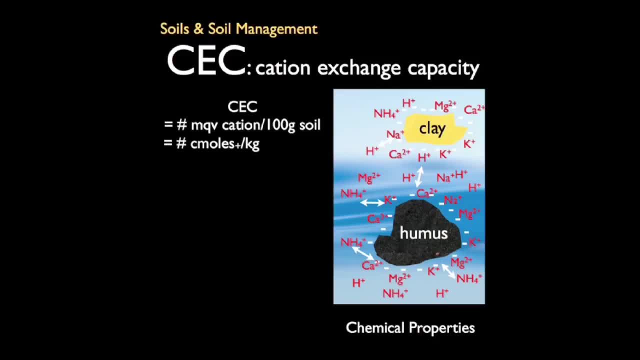 cations. This ability has been traditionally defined as the number of milliequivalents of exchangeable cations held by 100 grams of soil. A newer and preferred measurement of cation exchange capacity is expressed in centimoles of positive charge per kilogram of soil. 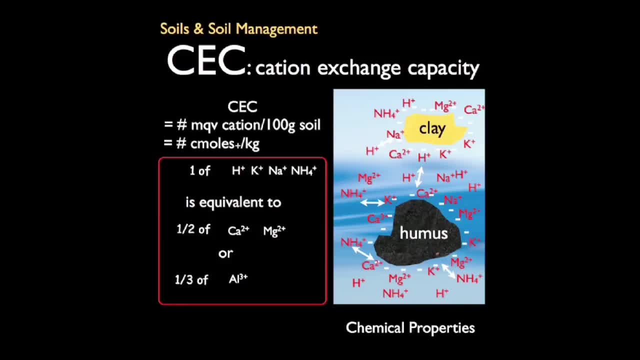 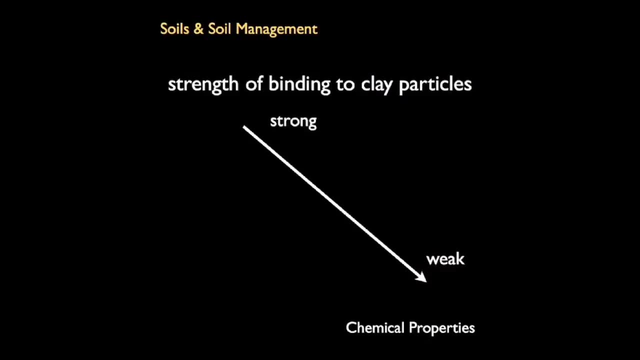 Milliequivalents were used to refer to the number of charges. Milliequivalents were used to refer to the number of charges exchanged rather than the number of ions, because different ions carry different amounts of charge. Not all cations are attracted to or held by the cation exchange capacity with equal energy. 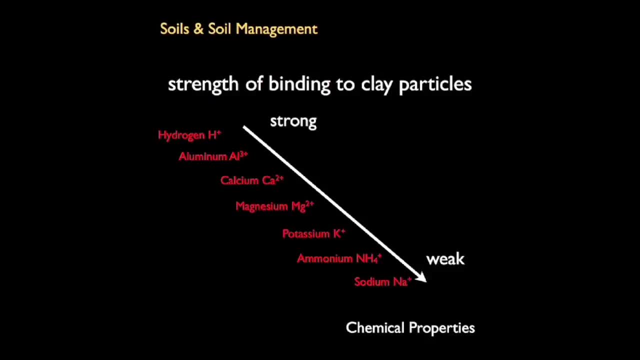 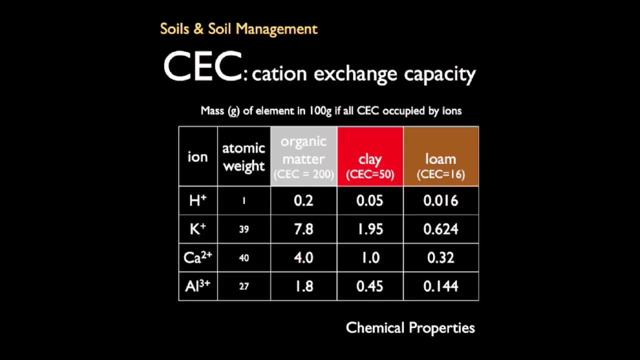 The strength varies as shown here. with hydrogen and aluminum bound more tightly than ammonium and sodium, Organic matter colloids typically display a cation exchange capacity. Organic matter colloids typically display a cation exchange capacity. They have a cation exchange capacity of 200, shown here in grey, whereas clays range. 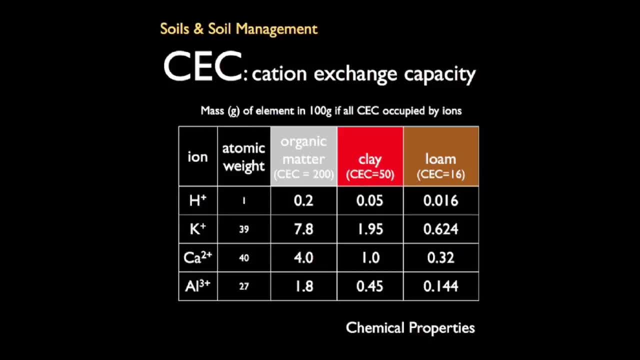 in CEC from approximately 10 to 100,, for example, shown here in red at 50.. An average loam containing 2 to 5 percent organic matter and 20 percent clay might have a CEC ranging from 14 to 20, shown in brown here as 16.. 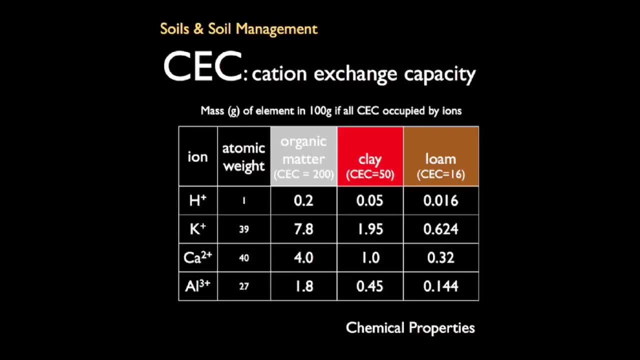 The numbers on this table are the mass in grams: grams of hydrogen, potassium, calcium and aluminum in 100 grams of soil. if all cation exchange capacities are occupied by ions, So organic matter with a higher CEC can hold more ions than low, as indicated by the higher numbers under that column. 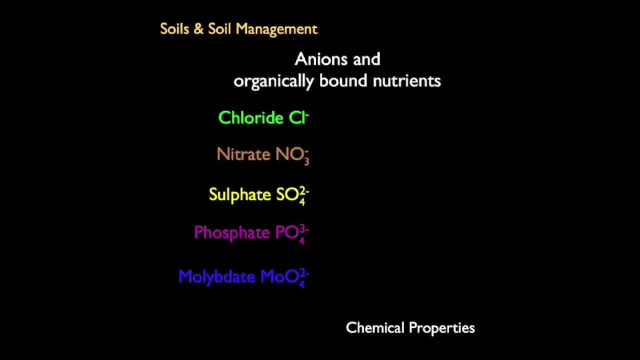 Now what about anionic nutrients such as nitrate, sulfate, phosphate, molybdate and chloride? Is there any anion exchange capacity that corresponds to CEC for these ions? Anions are indeed more subject to leaching than cations. However, clays, under some conditions and in 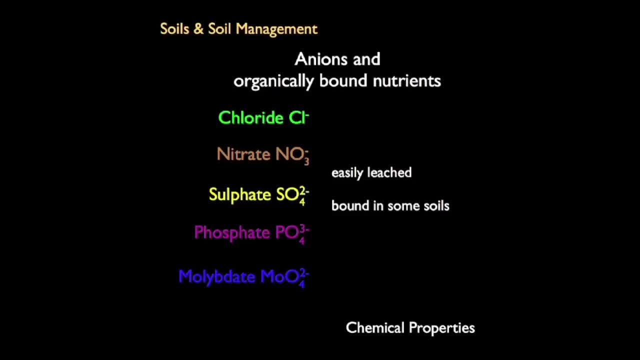 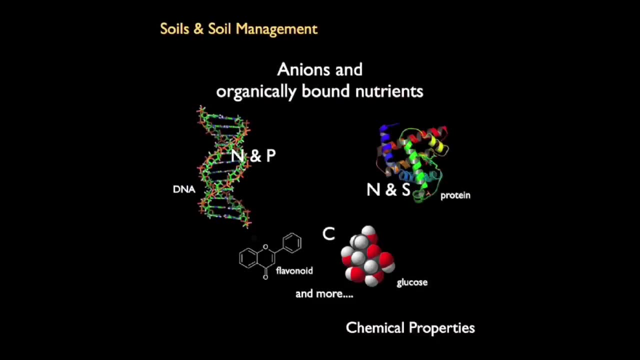 more neutral soils may act as agents of anion exchange, although the chemical details of these processes are not well understood. Much of these negatively charged nutrients, and particularly nitrogen, are locked up in more complex high-pressure and high-pressure organic material such as protein, nucleic acids and other compounds in soils. so the 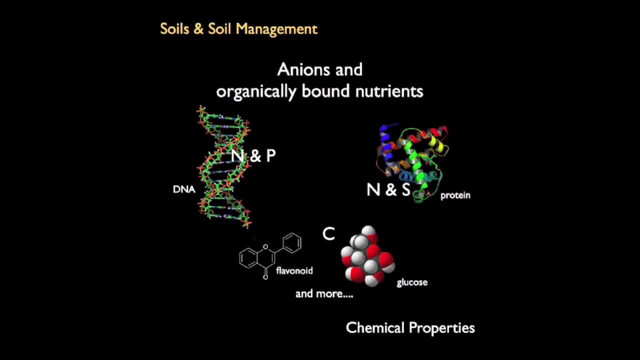 amount of nitrate present does not give much indication of the future availability of nitrogen for plants. Carbonate is unusual among soil ions in that it is exchanged through its equilibrium with carbon dioxide in the atmosphere. Now the pH of the soil solution or its hydrogen. 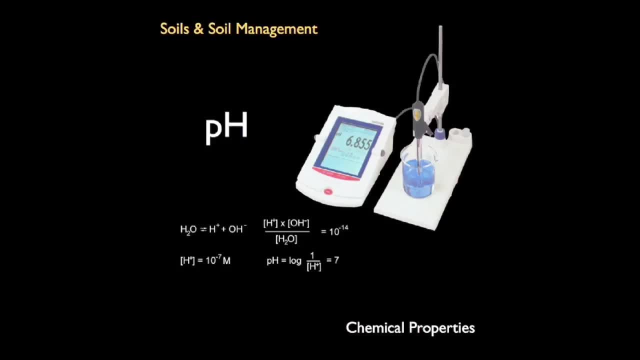 ion concentration can drastically affect the soil's nutrient storage capacity and availability of nutrients in the soil solution. Pure water is neutral because it has an equal concentration of hydrogen and hydroxyl ions. Only a tiny proportion of the water is dissociated and the hydrogen ion concentration is 10 to the minus 7th molar. pH is the log of the reciprocal 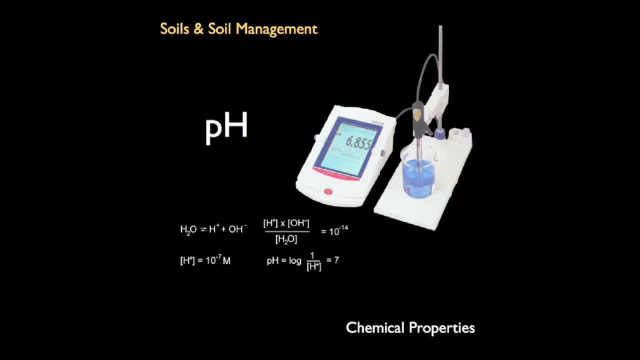 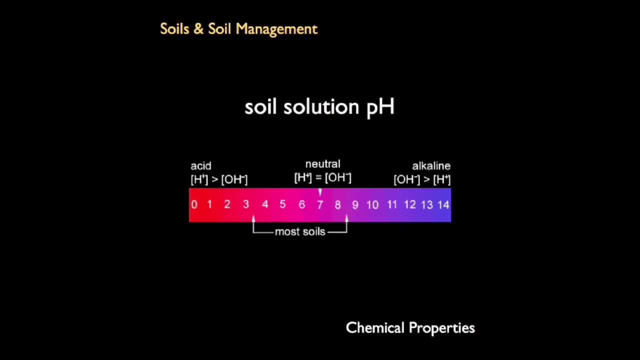 of the hydrogen ion concentration. So the pH of pure water is 7.. Below pH 7, there are more hydrogen than hydroxyl ions and the solution is acid. Above 7, there is an excess of hydroxyl ions and the solution is alkaline. The pH of the soil solution varies. 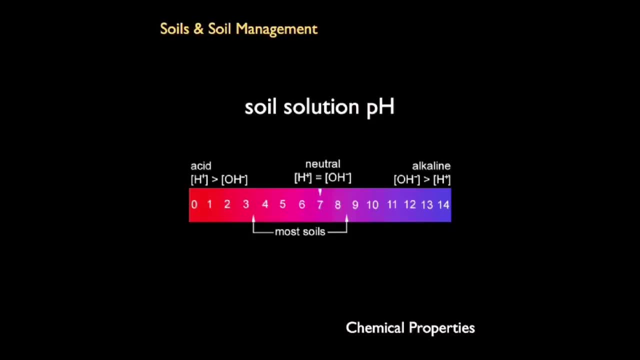 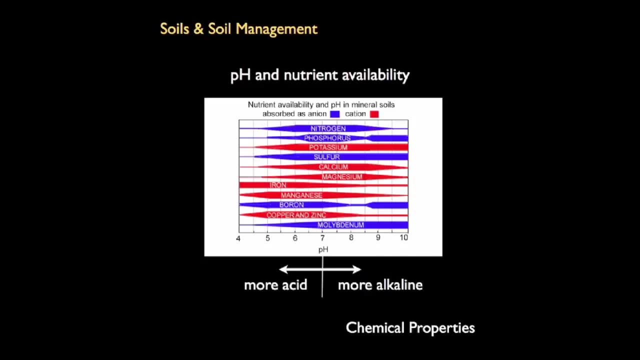 from 3.5 to 8.5.. The pH of the soil is often called the soil reaction. Since the beginning of the 20th century, soil scientists have been studying the effect of pH on the availability of nutrients, Although nutrient behavior is somewhat different. 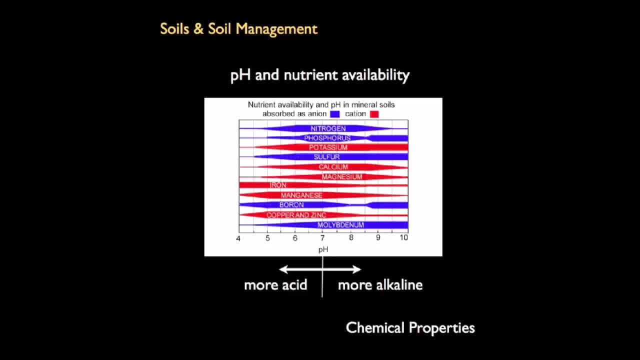 in each soil type, there are some general trends in nutrient availability in relation to pH As the soil becomes more acid. the availability of nitrogen, phosphorus, potassium, sulfur, calcium, magnesium and nitrogen will increase As the soil becomes more acidic. 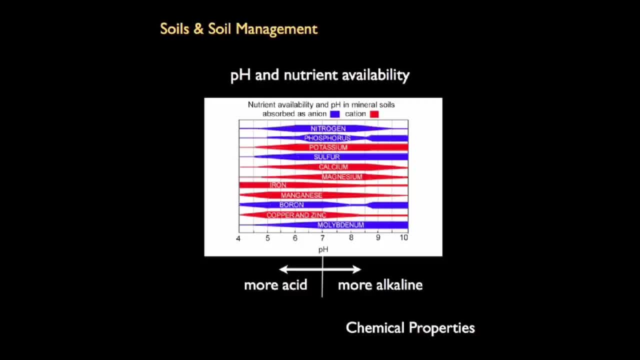 nitrogen and molybdenum drop off. Conversely, in basic soils, nitrogen, phosphorus, iron, manganese, boron, copper and zinc are less available. Therefore, the best window of nutrient availability for most plants in most soils is pH 6.5 to about 6.8.. And crop yields are